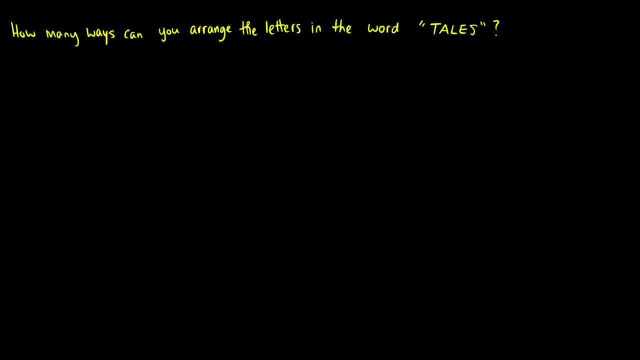 If not, I have videos in Discrete Math 1 explaining all the principles. So how many ways can you arrange the letters in the word tails? So we have five letters: t, a, l, e and s. We can swap letters around and have new order, For instance a, t e s. l is a method, So 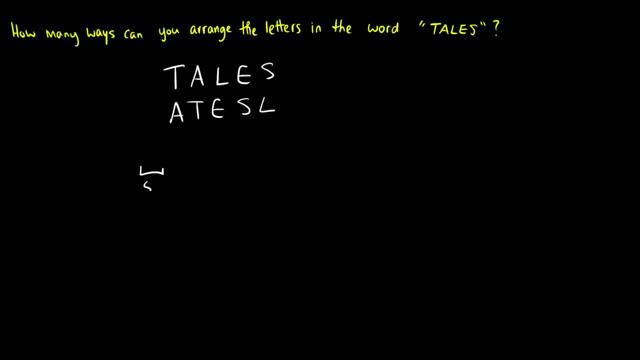 what we do is we take our first position and we say there's five ways to do the first letter. There's going to be four letters remain for the second position, three ways for the third, two for the fourth and one for the last. So this is 5 times 4 times 3. 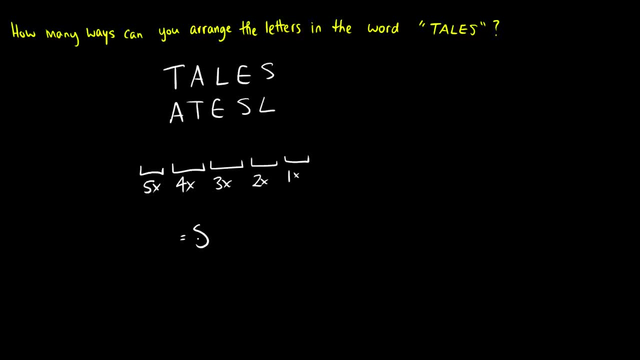 times 2 times 1, which is equivalent to 5 factorial. So again we can pick l for the first one. so we take the first and then check for it. That means in the second spot we only have a-t-e-s. 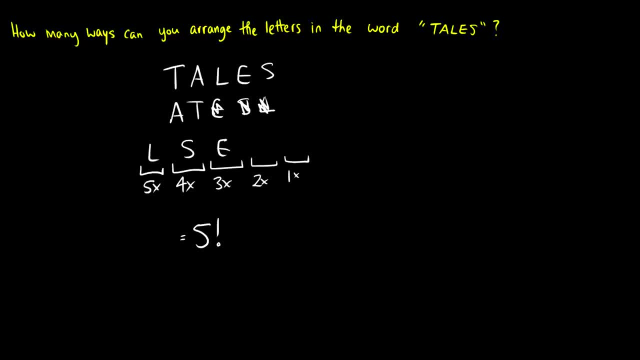 so we pick s, Then we have a-t-e, so we pick e, Then we have a and t left, so we pick a, and then we can pick t for the last one. So this is permutations, without repetition. Now we'll move on to another word. except this word is barbaric. So 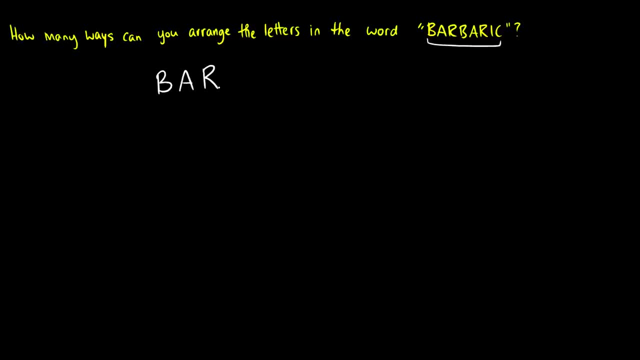 we have b-a-r, b-a-r, b-a-r, b-a-r, particularly maybe b-r and r, except then we come to another b, so we skin, compared to the six wheel, know that this wordб. So I'm just going to list that B below. 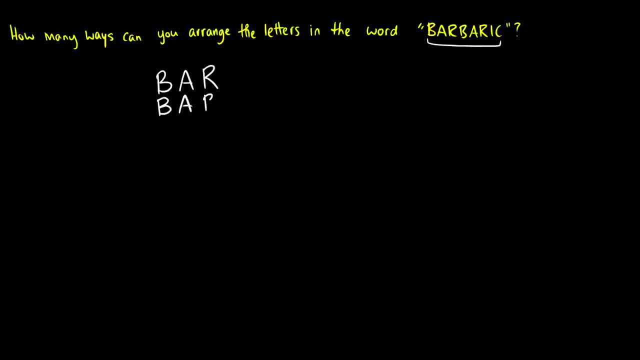 And then we have another A, Then we have another R, Then we have an I and a C. So this is a little bit different, because, well, first of all let's order them. So we have eight factorial spots to fill. 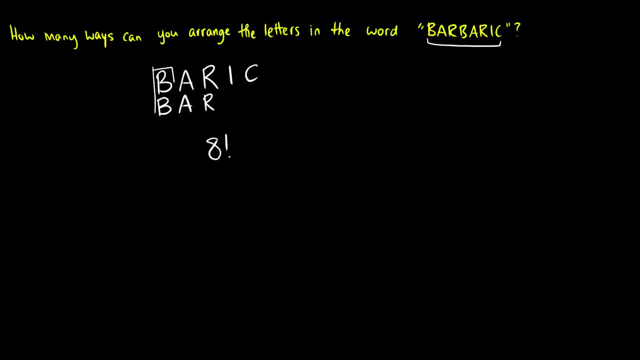 But the B's are similar, the A's are similar and the R's are similar. So this means, if we make say BBAARRIC, in this case we might have one alteration where this is B1, B2.. 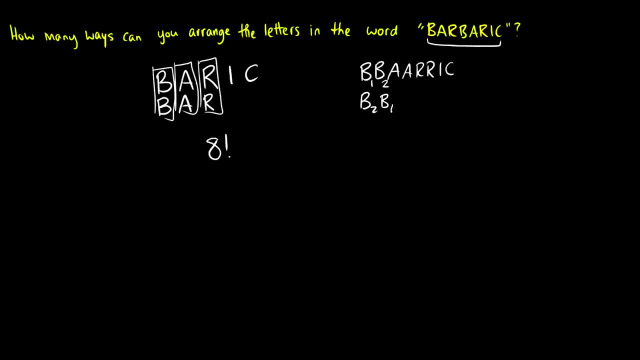 And we might have another one where this is B2, B1. So we're counting every pair of B's twice. So we have to divide by 2 factorial for the B's. There's also going to be situations where we're counting the A's. 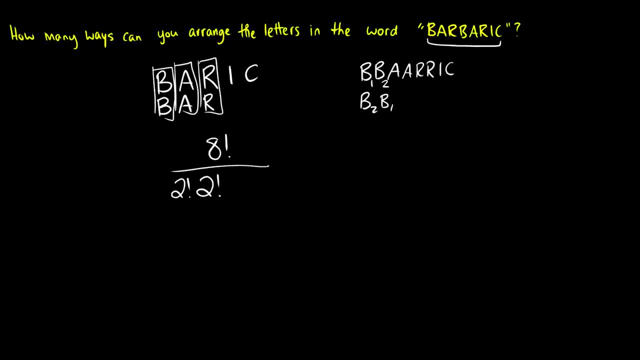 So we're going to do that twice. So we divide by 2 factorial for the A's And we divide by 2 factorial for the R's, So we get our final answer here of 8 factorial over 2 factorial times 2 factorial times 2 factorial. 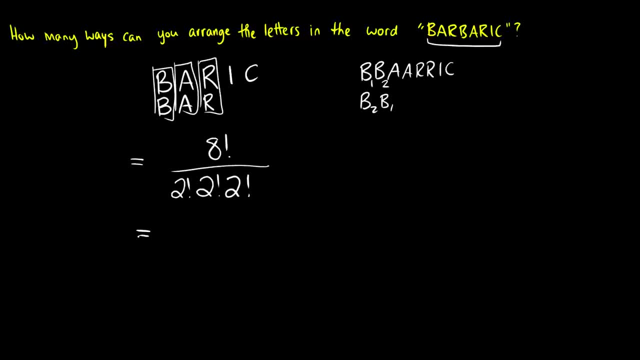 Now we can write this as a multinomial coefficient, So we can write this as 8 with 2, 2, 2, 1, 1.. That can be represented the same way, since we're really also dividing by 1 factorial i's and 1 factorial c's. 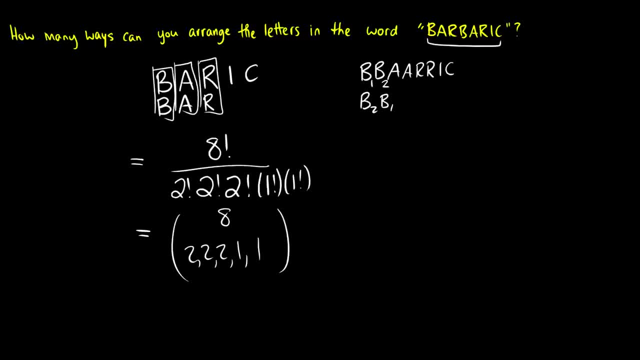 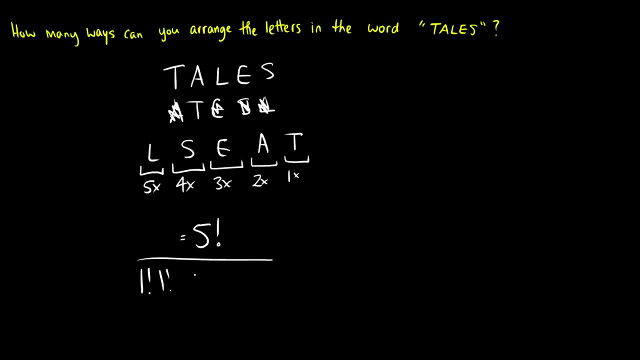 Except there's only one of them and 1 factorial is just 1, so we leave it out of the denominator, But it's good to mention that really in this previous question it's 5 factorial over there's 1t, 1a, 1l, 1e and 1s. 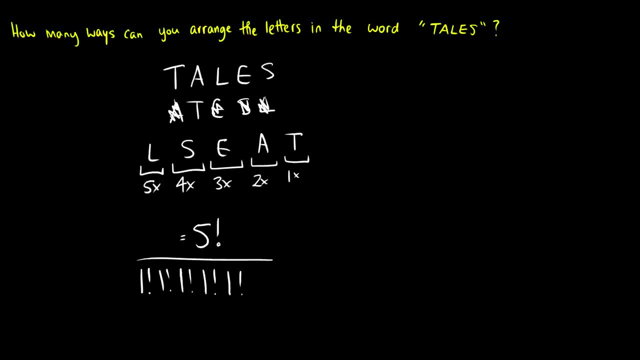 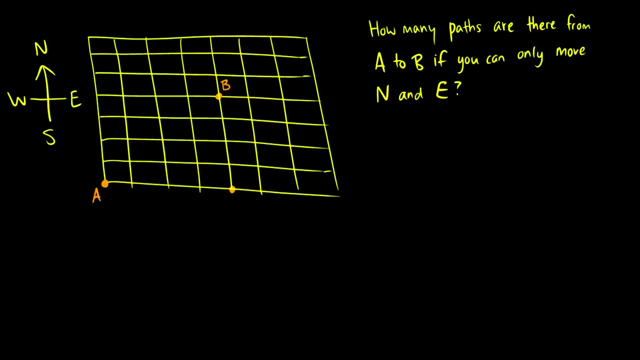 But that's not necessary. So that is another permutation question when we have repetitions in them. So here's a fun question And this is pretty important. lattice paths are interesting and this question is sort of crucial to a topic coming up in the next video. 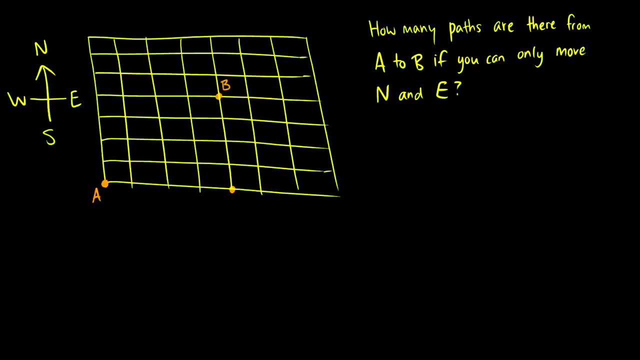 So this is a grid and we want to go from point A to point B, going only north and only going east. So we start here at 0, 0, and we need to go 1,, 2,, 3, 4 to the right and 1, 2, 3, 4 up. 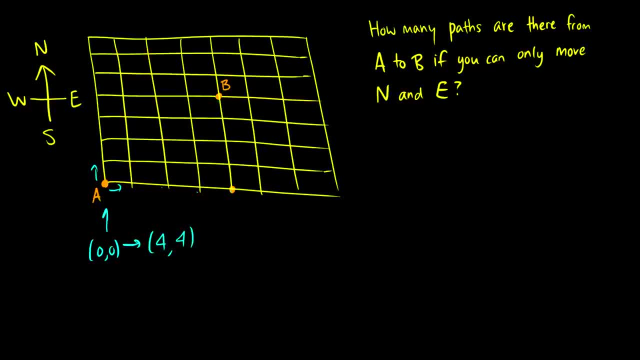 So we're going from 0, 0. To 4, 4.. Okay, so this is kind of like making a word. So when we go 4 to the right, what we're doing is we're going east, east, east east. 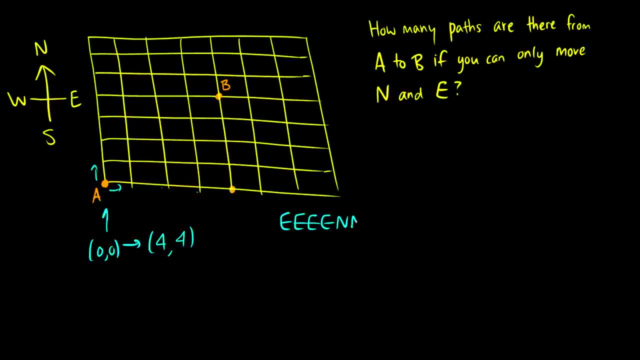 And then we need to go north, 4. So we have n, n, n, n, And we can rearrange these so we can get a different path. So, for instance, I have north east, north, north east, north east. 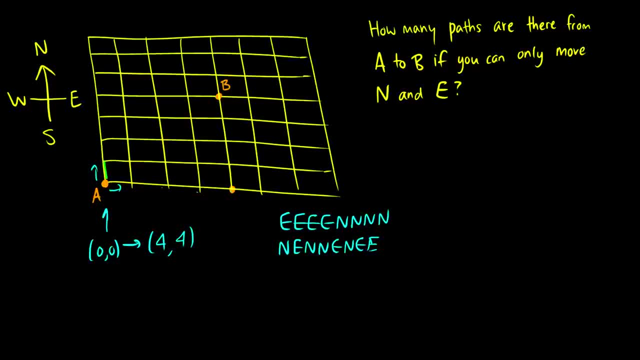 So let's draw that one. We go north, we go east, we go north, north, east, north, east, east. So that's a path. So what we can do is we can just figure out how many ways we can arrange these letters so that they're distinct paths. 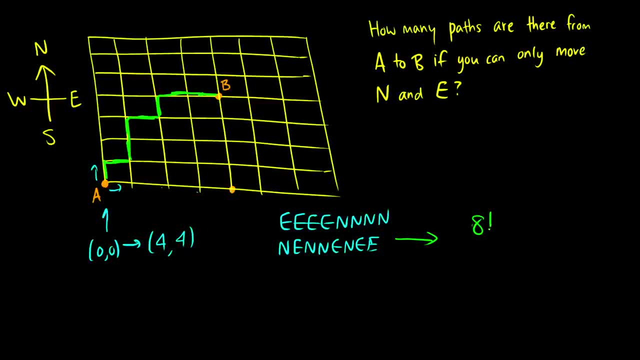 Well, we have 8 total letters, so that's 8 factorial over. well, we have 4 n's, so we divide by 4 factorial. And we have 4 e's, So we divide by 4 factorial. 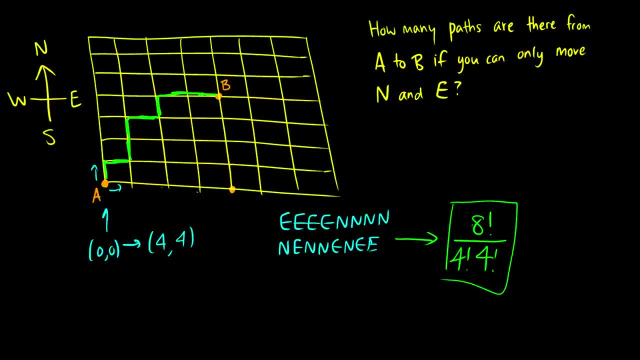 So this is the solution: from 0, 0 to 4, 4.. Okay, so that's one specific example. Now let's make this a little bit more general. So we want to go from a, b to c, d. 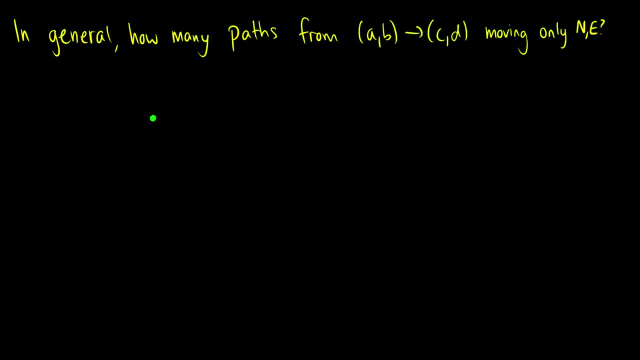 Okay, so that means we pick some arbitrary point- a, b, and then there's some points somewhere else- c, d- And we want to know how many way we go up And how many ways we go right. So we can do this using any method we want: pictorially, but really, what's the distance? we're changing in x values. 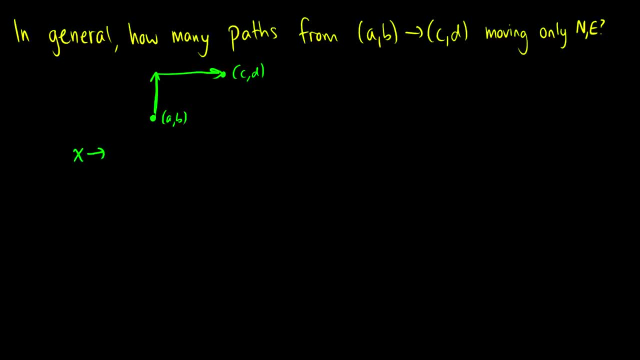 So the x value is going from a to c. So the distance is c minus a for the x's. call that delta x, Our change in the y direction. how many ways we go north? We go from b to d. 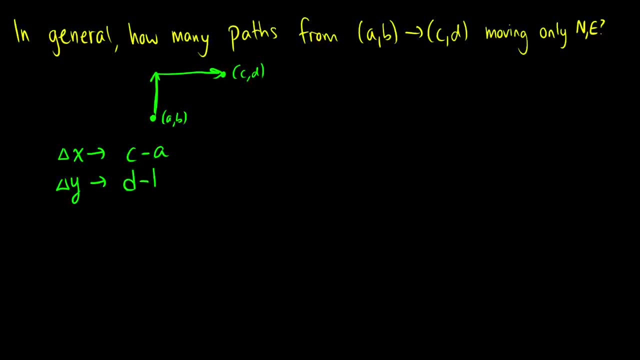 So the change in y is going to be d minus b. So we're going c minus a to the right and d minus b to the north. So how many total ways or how many total moves are there? How many total norths and easts are there? 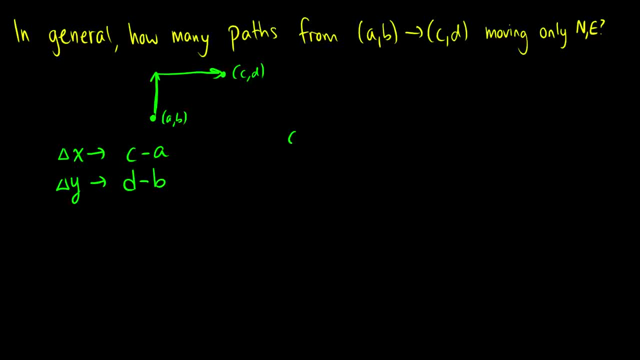 Well, there's going to be c minus a moves to the right, plus d minus b moves north. So that's the total amount, So that's our factorial: c minus a, plus d minus b, factorial. And then we want to divide by how many of the same letter there are. 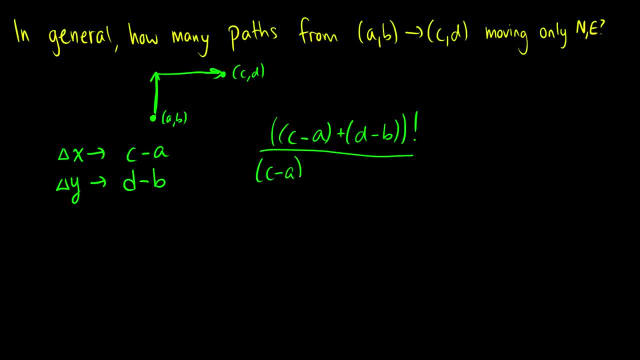 So there's going to be c minus a easts and there's going to be d minus d minus b norths. So this is the solution to the general question. This may look a little bit confusing, but we can just say that m is equal to c minus a. 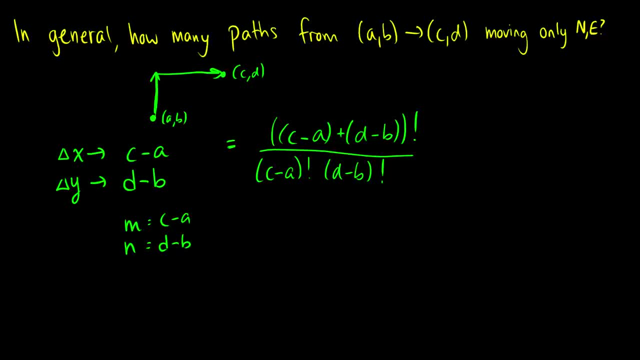 n is equal to d minus b. So this is our delta x here. This is the. Actually, I should write down the number of easts and the number of norths is equal to m. So this is really just m plus m plus n factorial over m factorial, n factorial. 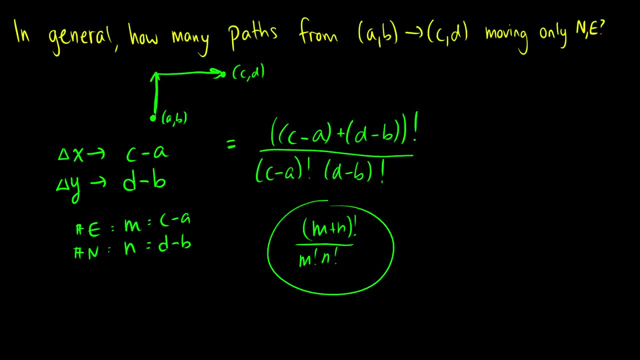 And this is a general equation you can use for any lattice problem. In fact, even if what we're doing is we're going from ab to cd, going down and left, we'd still get sort of a proper answer. Of course, realistically, we know that the answer is zero if we're going down to the left. 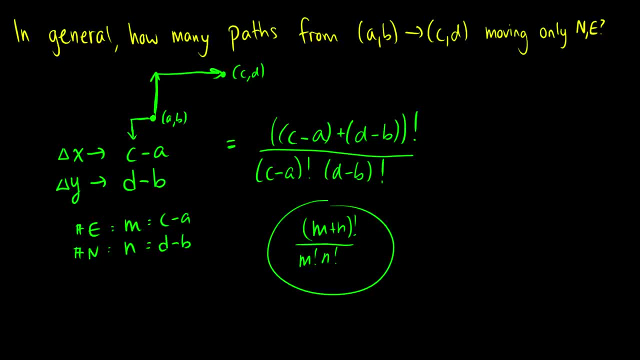 But you know what. Play around with it. See what happens. So that is some more permutations with repetition. What's interesting about this is that this can actually be written as a combinatoric problem where it's m plus n choose m, Or we can write m plus n choose n ways. 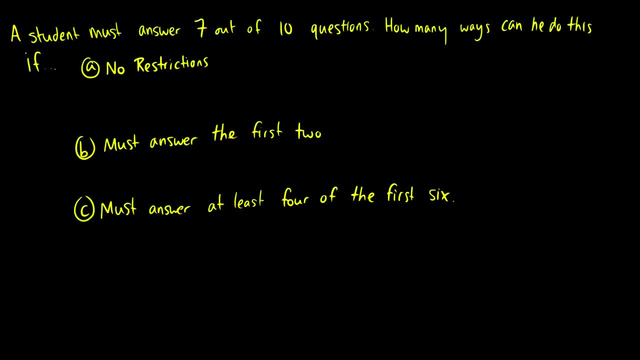 That's the same thing, All right. So here's a nice combinatorics problem. So a student wants to answer 7 out of 10 questions on a test. How many ways can he do this if there are no restrictions on which questions he answers? 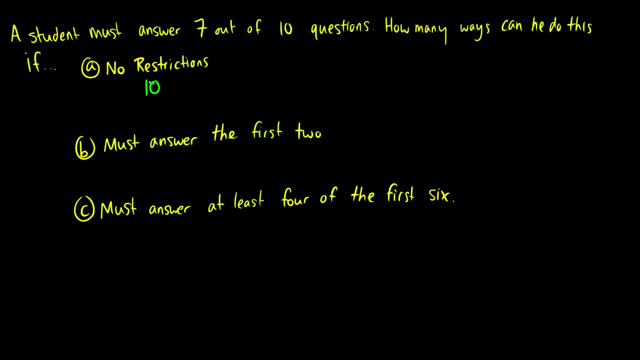 Well, there's 10 questions total and he has to answer 7 of them. So let's just 10, choose 7, which, if you don't remember the formula, this is 10 factorial over 7 factorial. So if we have n, choose k. 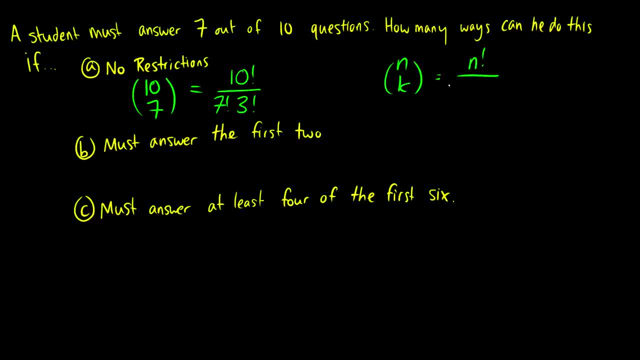 this is equal to n. factorial over k factorial times, n minus k factorial, It's the same thing. So n over k is the same thing as n choose n minus k, Because if you expand it out you'll get the exact same equation. 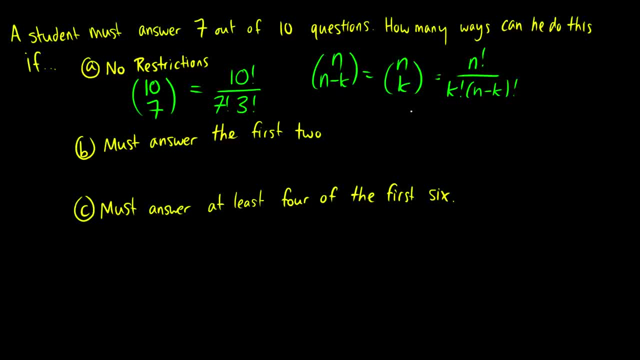 So this is an important thing to remember. So if you can remember this and put this in your memory forever, you're going to be a lot happier on your exams if you take this course in real life. Okay, so what about if the student must answer the first two questions? 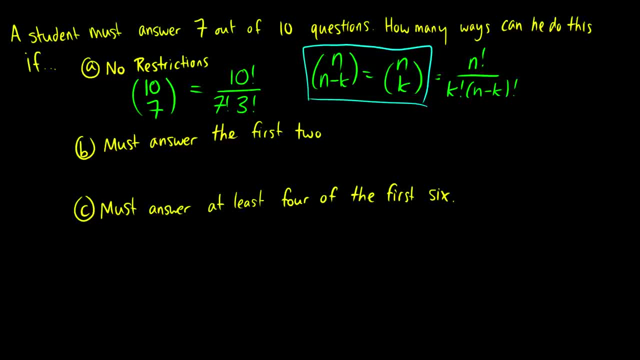 Okay, so what this really means is that he's taking the first two and he's choosing both of those, And then he has the remaining eight questions and he has to answer seven of them, but he's already answered two, So he has to pick five of the remaining questions. 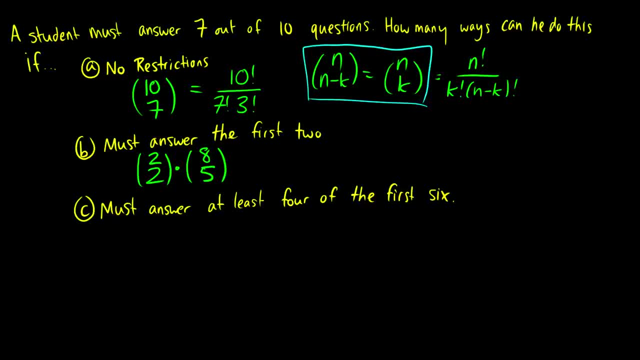 So 2 choose 2 is the same thing as 1.. So this is 1 times 8 choose 5.. So it's really just a question of saying how many ways can he answer five questions out of the last eight. So this would be 8 choose 5.. 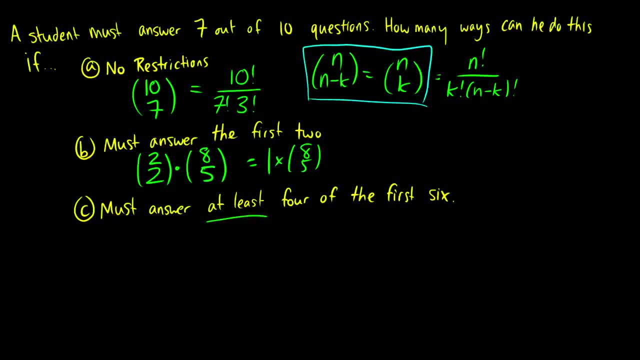 Now what if he must answer at least four of the first six questions? Well, what this means is that he can choose four out of the first six and then he can choose out of the remaining four. he can choose three questions. So basically, he's splitting it up into two categories. 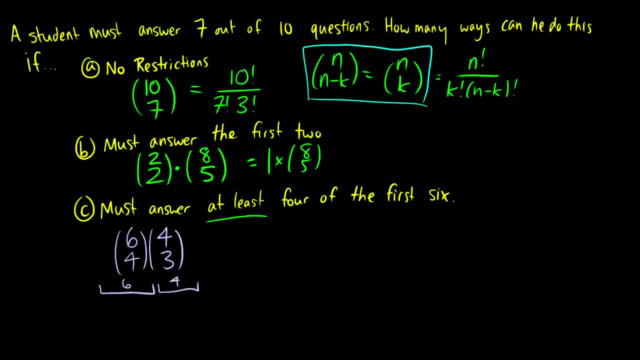 Here's six questions, the first six questions and here's the remaining four questions. This one: he picks the first, the second, the fourth and the fifth, and then, in the second part, he picks the eighth, the ninth and the tenth. 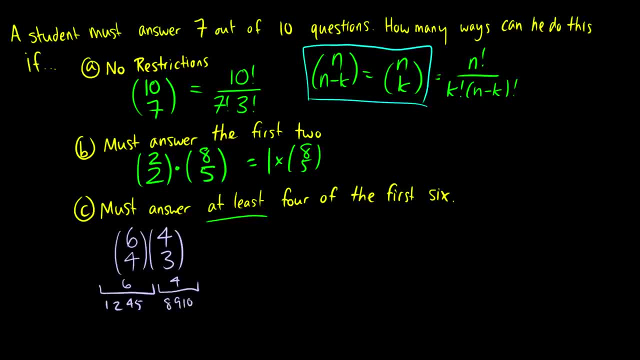 So those are the questions he could answer. So we multiply them because the order could change or not the order, but the selection could change for the last four questions. So instead of 8, 9, 10, we might have 7, 8, 10.. So this is why we multiply. 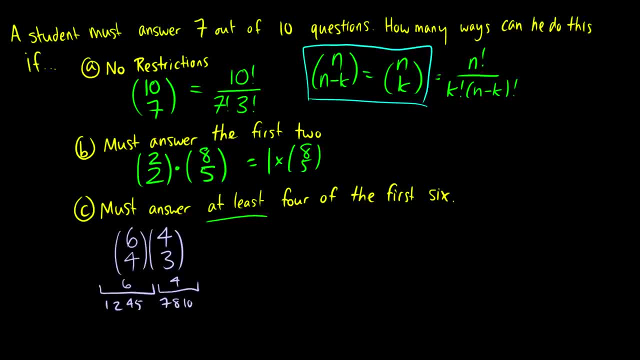 Now, the question didn't ask if he only answered four. they said at least four. So we also have to add the situation where he answers five out of the first six questions, which means he only answers two out of the remaining four, And then if he answers all six of the first six questions. 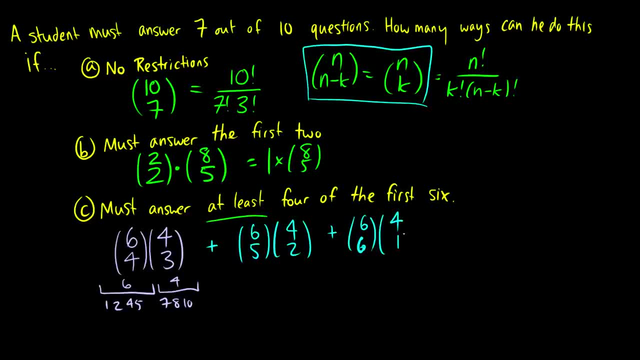 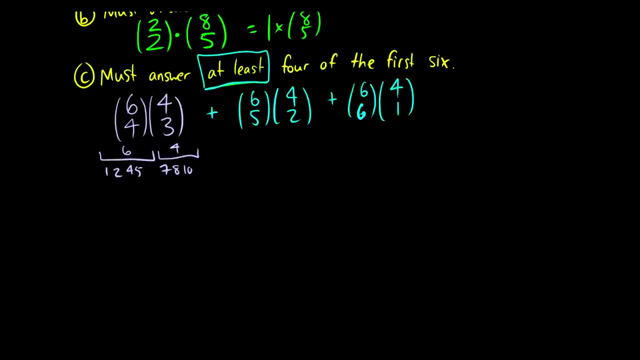 then he can only pick one out of the last four. So this would be your solution to answering seven out of ten questions if he must answer at least four of the first six. So this is a little bit neater, a little bit more complicated, I guess. 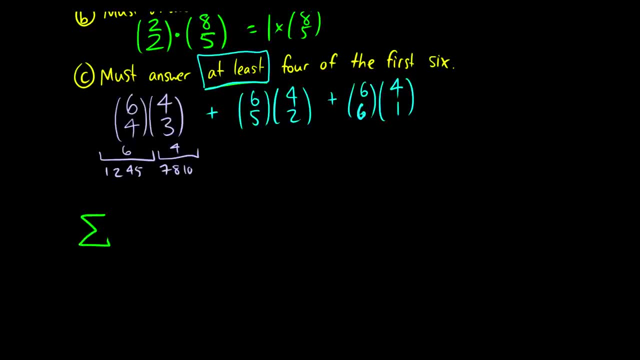 We could write this as: the sum, as i equals four to six of six. choose i times four, choose. how do we want to do this? If i is equal to four and it's going up, then we want to do this like: hmm, I might want to pick better numbers here. 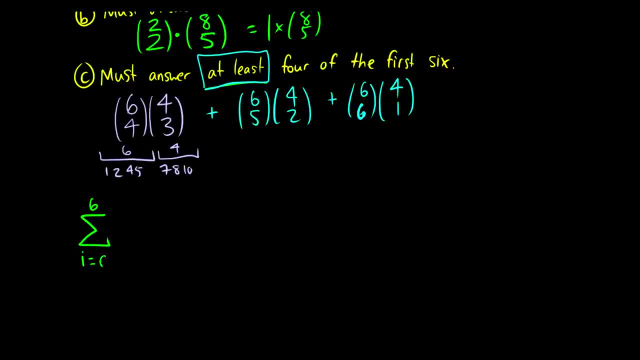 Let's pick: i equals zero, and we'll go six: choose four plus i. four, choose three minus i. That looks a little bit nicer, And this will be: i equals zero to two. So I mean, even for me it takes a little bit to figure out. oh, how do I write this? 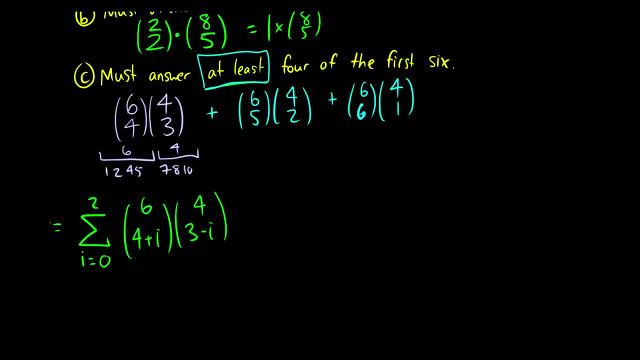 How do I write this in sigma notation? But this is just equal to this, And you're going to be seeing a lot of sigma notation in this course, so you might want to get used to this. I'll probably reintroduce it when I need to. 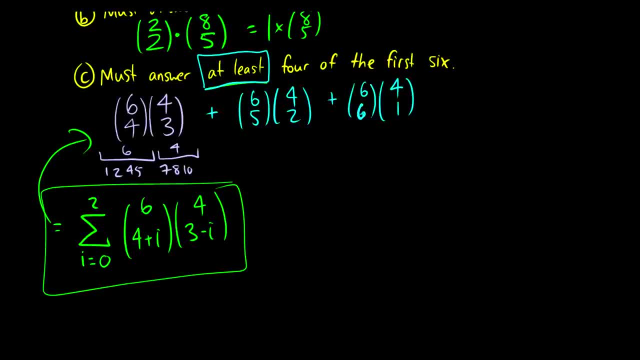 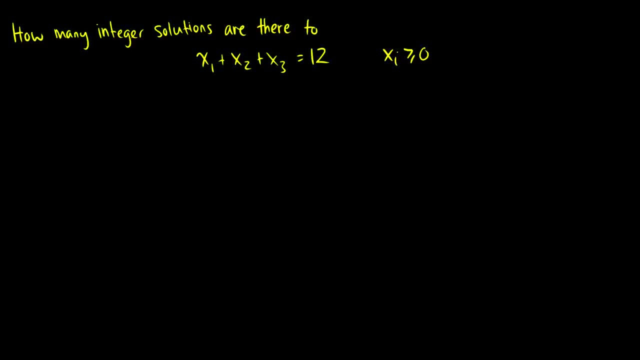 but this is just a nice concise way of writing this answer. All right, Now we've dealt with combinations without repetitions, so let's jump into combinations with repetitions. Here's a question I did, and I even put on there my own final that I wrote for the first course. 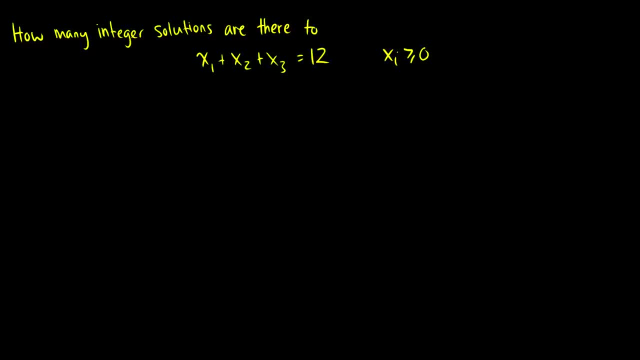 which you can do at trevtutorcom. If you go to discrete math, there is a final for discrete math, one that I made with the solution key. So here's a question that was similar to one on there: How many integer solutions are there? 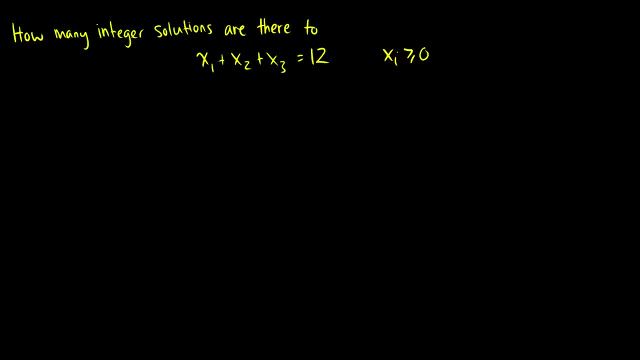 to x1 plus x2 plus x3 is equal to 12?. So what we're saying here is that we have three distinct bins: We have our x1,, we have our x2,, we have our x3, and we want to distribute 12 items into them. 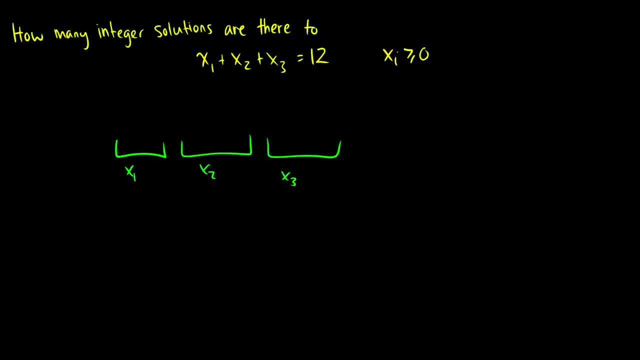 So the bin can have zero or more items. so we might put- I don't know, let's put 1, 2, 3, 4, 5, 6 in x1.. We put 2 in x2,. 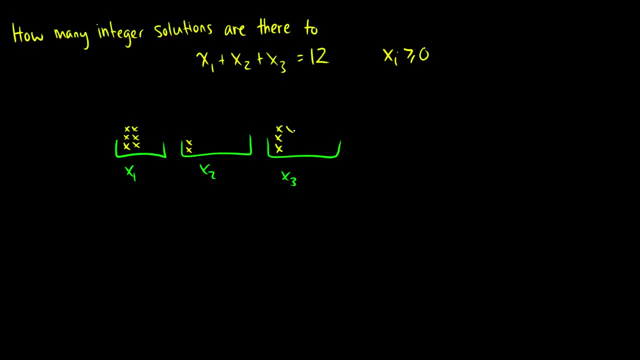 and then we put 4 in x3.. So that's one way that we can do it. So here's the question: How do we do this into a combinatorics problem? Well, what we do is we line up 12 items. 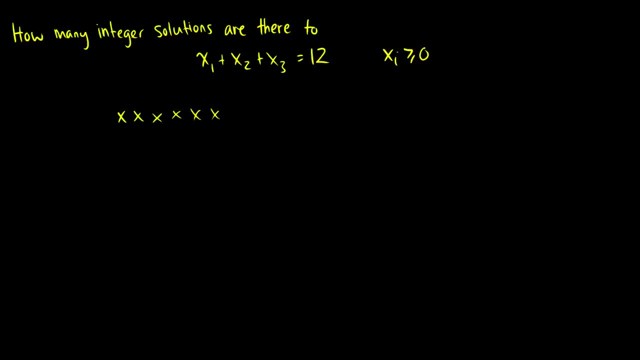 So there's 6,, 7,, 8,, 9,, 10,, 11,, 12.. And what we do is we insert separators. So because there's three bins, we have to insert two separators. So we could put them here and here. 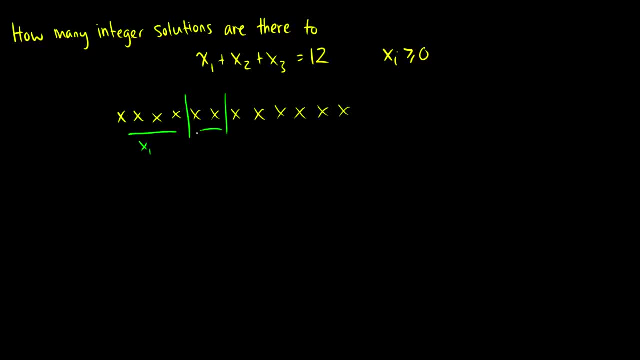 So now this right here is our x1.. This is our x2.. And this is our x3. Now what we can also do is we can put them both, say here and here, So we have nothing in x1,, nothing in x3,. 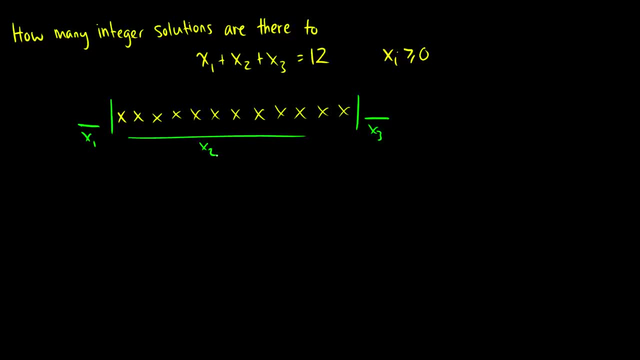 but we have everything in x2.. So really, what we're doing here is we're not picking 12 objects or choosing 12 objects. We're actually looking at 14 spots and we're going to put a divider into two of them, So this is actually equal to 14. choose 12. 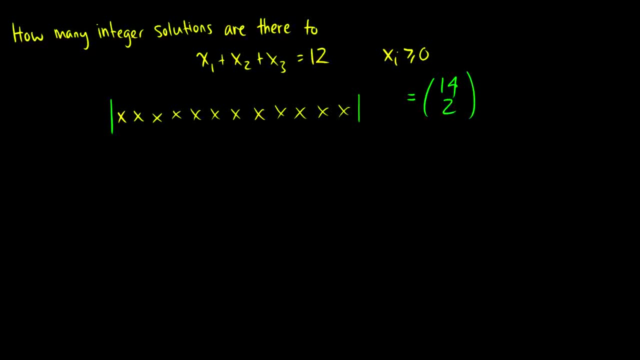 or I should say 14, choose 2, because we have 14 spots and we are putting in two dividers. So there's another way to look at this and that would be that we have 3 bins plus 12 objects. We subtract 1. 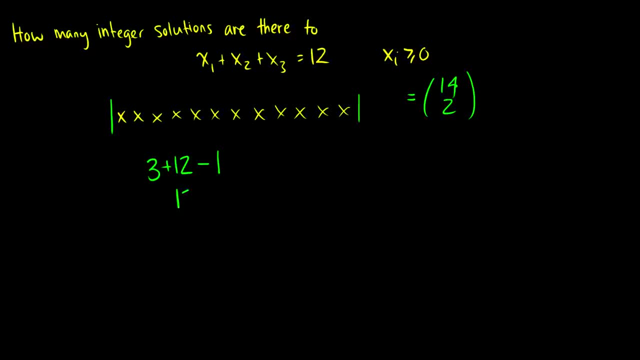 from the amount of bins we have and we choose 12 of them. So this is the same thing. This is 14 choose 12, which is the same thing as 14 choose 2.. And I'll give you a general formula for this. 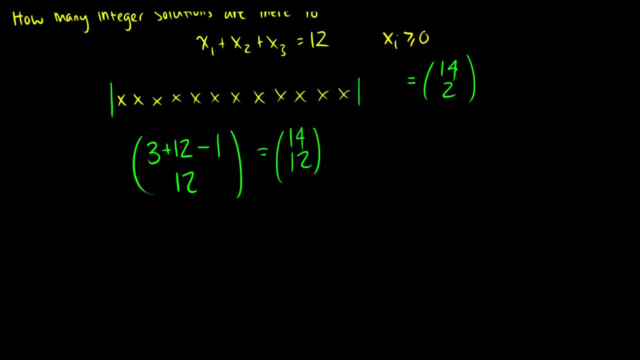 because it's very important to have the general formula if you don't understand the ideology behind it. And that is, if we have x1 plus x2 plus all the way to xn and we choose k objects, then this is equal to n plus k minus 1. choose k. 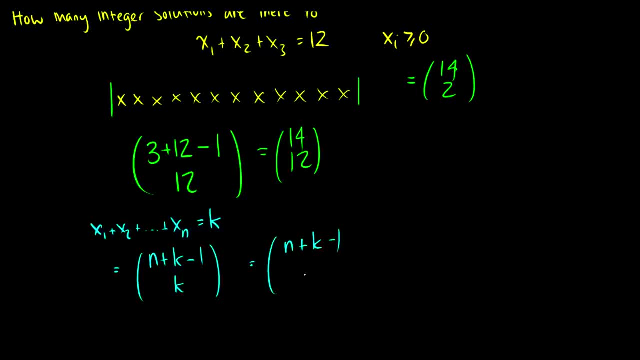 which is the same thing as n plus k minus 1. choose n minus 1.. So that's two ways of looking at things. Our n in this case was 3, our k was 12, and we subtract 1, so we get 14. choose 12.. 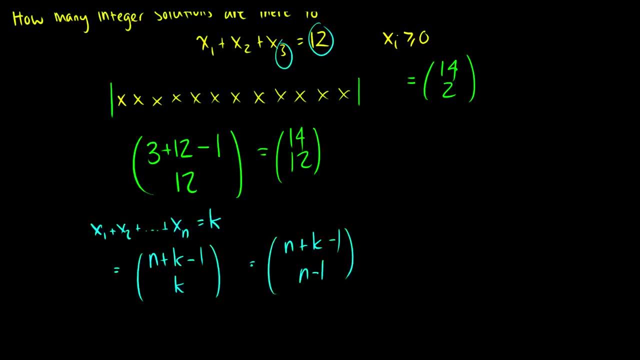 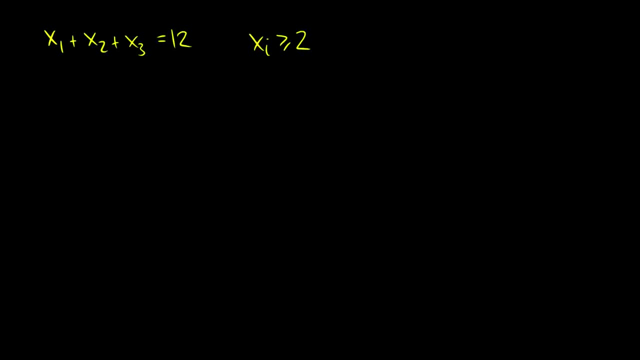 That's what I taught in the first video on combinations with repetition. What I didn't teach- which I didn't put on the exam anyway because I'm mean- is what happens when we require that certain bins need two objects, At least two objects. 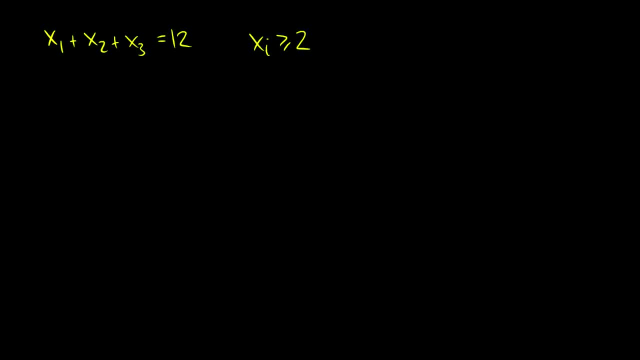 Well, we make some substitutions. So we're going to say that x1 prime is equal to x1 plus 2.. So we're just going to rewrite the problem. we want to shift it to an equation where xi is greater or equal to 0. 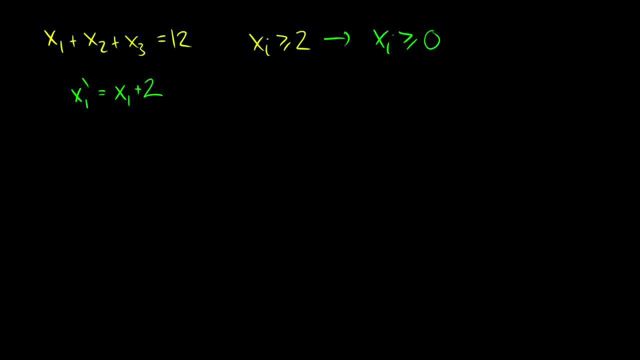 because we know how to deal with that. So we're just going to redefine the variables and make that a problem. So this x1 can be 0 or greater and it's going to have at least 2 in x1 prime because we're adding 2 to the bin. 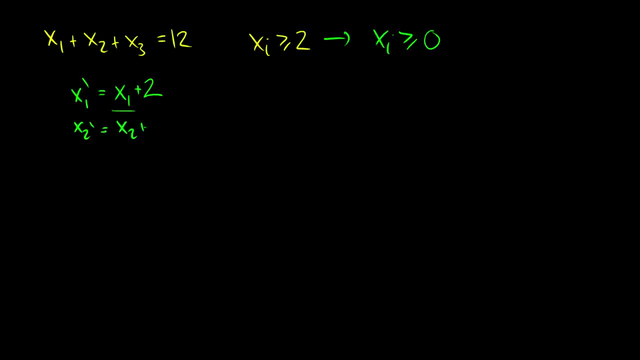 We can do this with x2 prime, so this will be x2 plus 2 and x3 prime will be x3 plus 2.. So we could rewrite this equation here. So we have x1 prime plus x2 prime plus x3 prime. 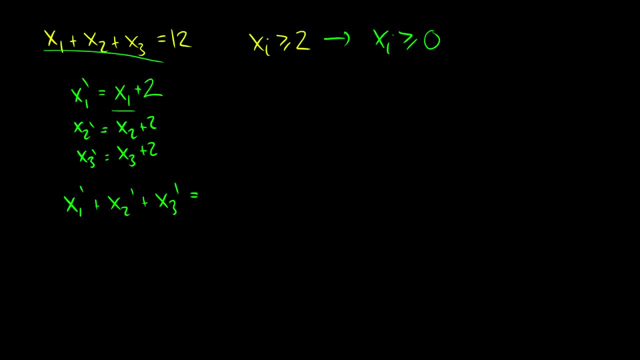 is going to equal. well, we have. I should write this: we have 12 here, but we have a plus 2 here, so we're going to have to subtract it from that, because x1 prime is x1 plus 2, but we only have an x1 up here. 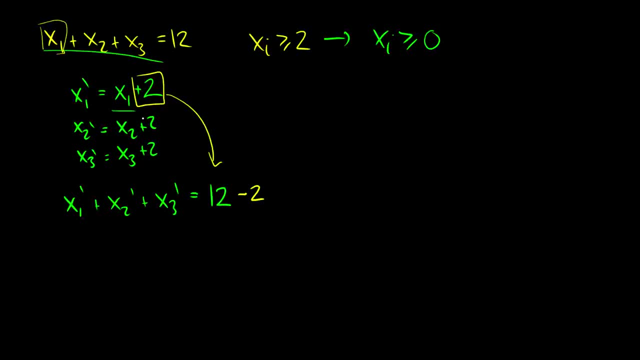 We're missing the plus 2, so we subtract it from the right side And similarly we do this with the other 2. this will be minus 2 minus 2 minus 2. so then we get x1 prime plus x2 prime plus x3 prime is equal to 6. 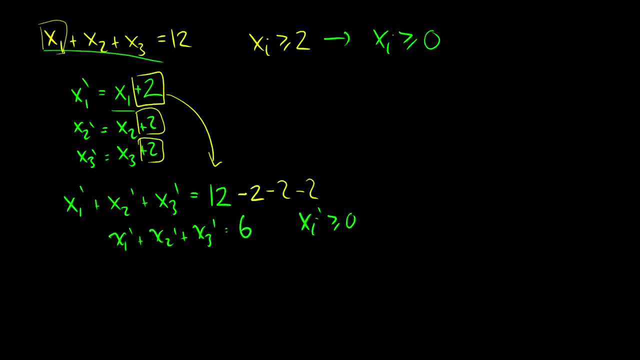 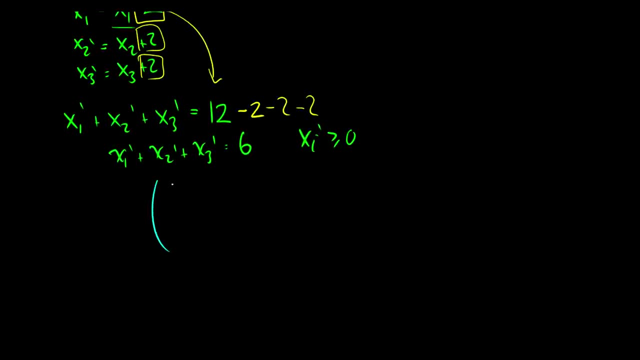 where all of our xi primes are greater or equal to 0. And now we just solve in the exact same way. We take: well, there's 3 bins and we're choosing 6. we subtract 1 and that's choose 6, so this is equal to. 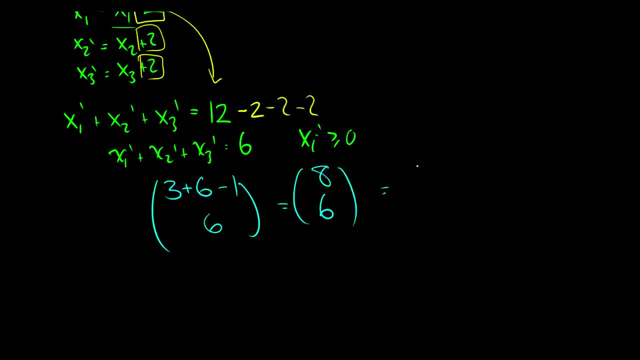 8 choose 6 or similarly, 8 choose 2: Same problem. we've just redefined some variables a little bit. You'll be seeing this when we do inclusion-exclusion, because there's some good questions you can do with this. So keep this one in mind. 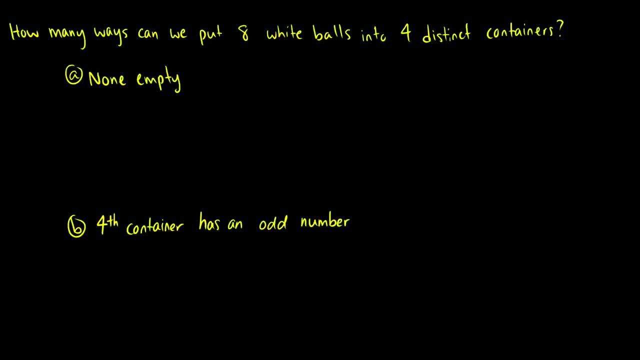 And finally, we just had some integer solution problems, but we can also have word problems that are combinations with repetition. So how many ways can we put 8 white balls into 4 distinct containers where none of them are empty? Well, we have 4 distinct bins. 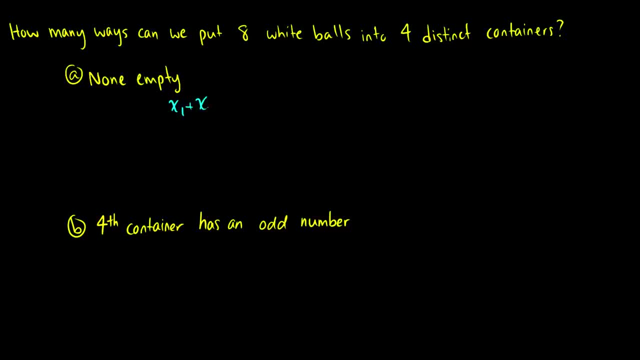 so that's our x1 plus x2 plus x3 plus x4, and we have 8 balls to distribute. So this is just this equation, and we know how to solve this equation. It's going to be 4 plus 8 minus 1. 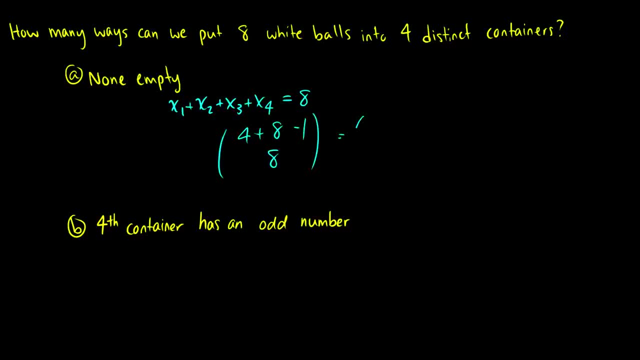 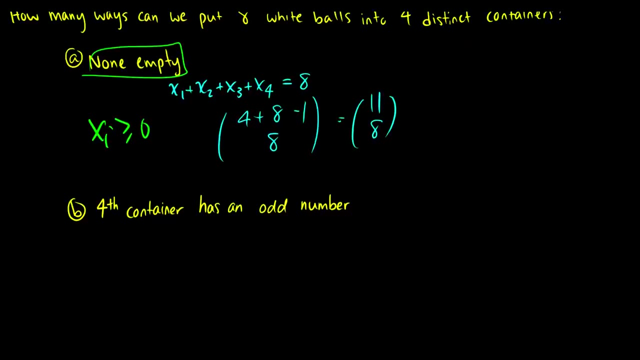 choose 8, which is the same thing as 11 choose 8.. What's important to remember in this example is that none of them are empty, so our xi's are greater or equal to 0 here. This one's a little bit more challenging. 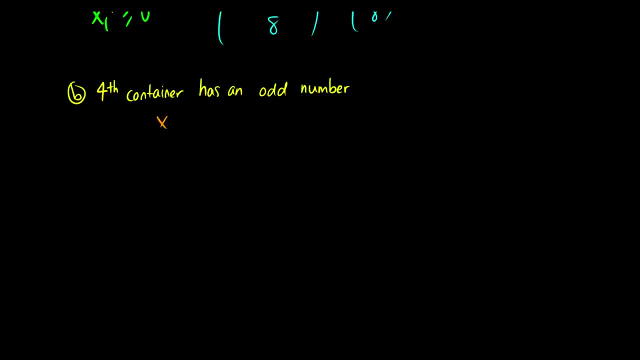 So we have the same equation here: x1 plus x2 plus x3 plus x4 is equal to 8. but we have a restriction: x4 has to be an odd number. So x4 is going to be 1 or it's going to be 3. 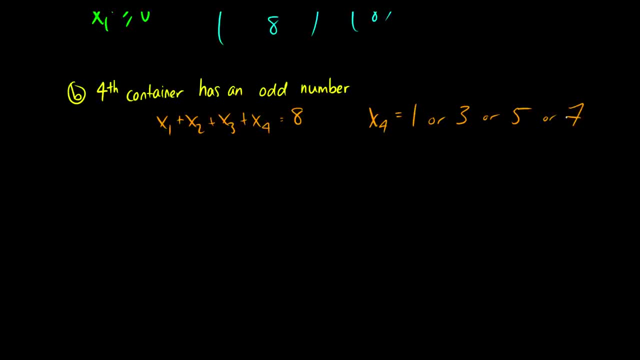 or it's going to be 5, or it's going to be 7.. So we have 4 questions to solve here. So we have the case where x1 plus x2 plus x3 plus 1 is equal to 8, because x4 is 1.. 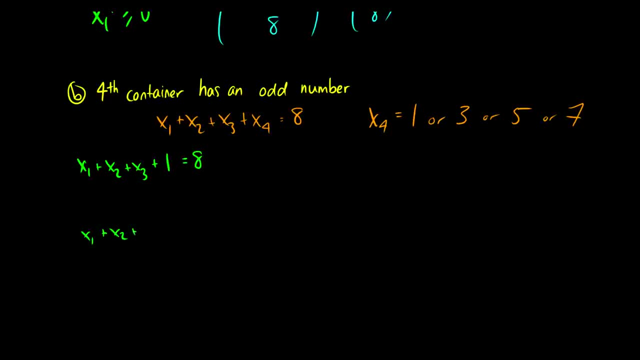 We have the situation where x1 plus x2 plus x3 plus 3 is equal to 8.. Then we have the situation where plus 5 is equal to 8 and plus 7 is equal to 8. So we have to add all these up separately. 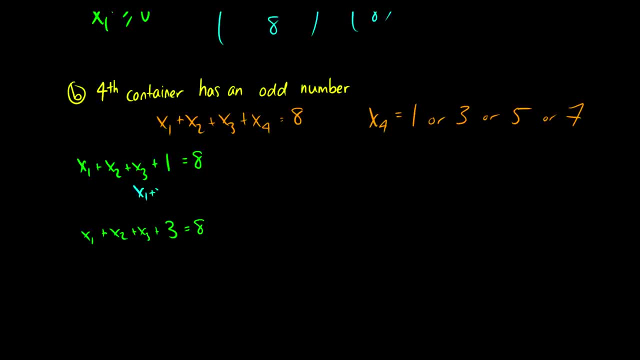 So this just becomes: x1 plus x2 plus x3 is equal to 7, which we know the solution by now. I'll just do it shorthand. So 3 plus 7 minus 1 is 9.. Choose 7. This one. 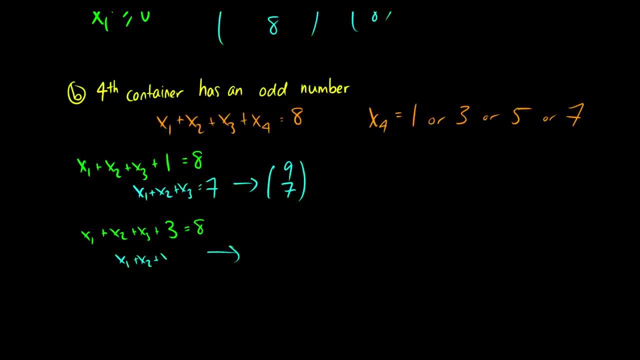 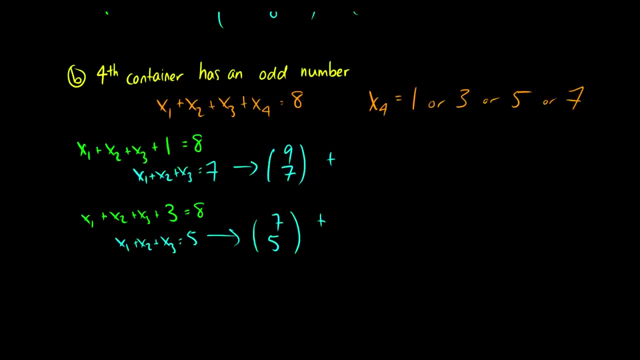 is going to be: x1 plus x2 plus x3 is equal to 5.. So 3 plus 5 minus 1 is 7.. Then we choose 5. And by now you can probably see the pattern. So you can guess that the next one is going to be: 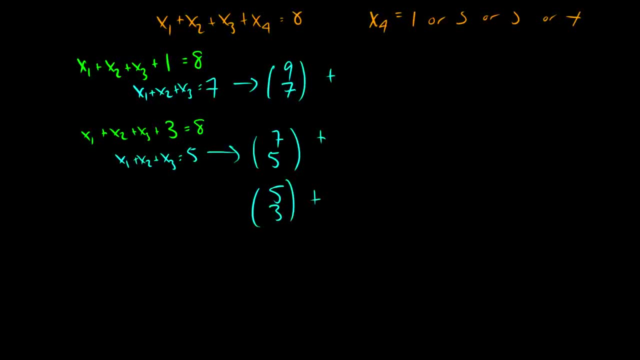 plus 5, choose 3, and the last one is plus 3, choose 1.. And that would be the solution where the last bin has to contain an odd number. You can verify these yourself, but normally if you see a pattern like this, it's: